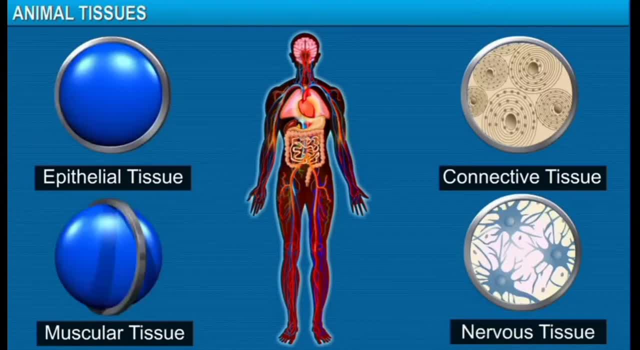 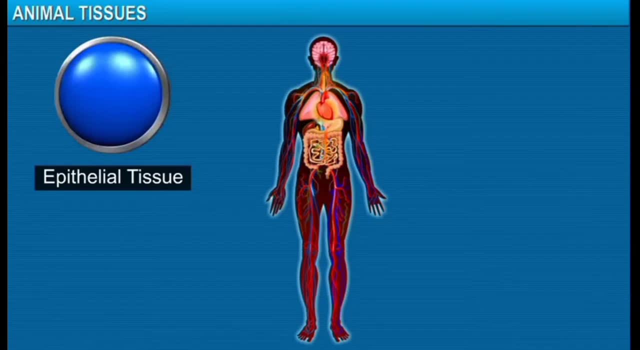 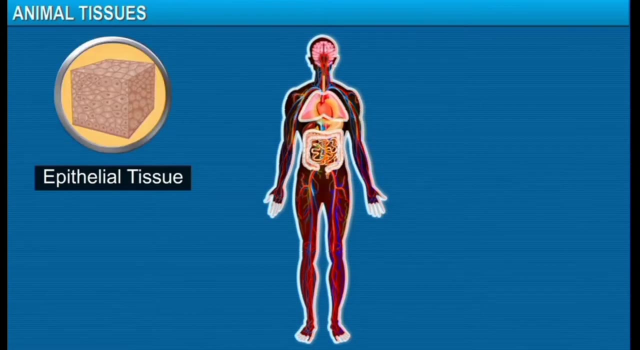 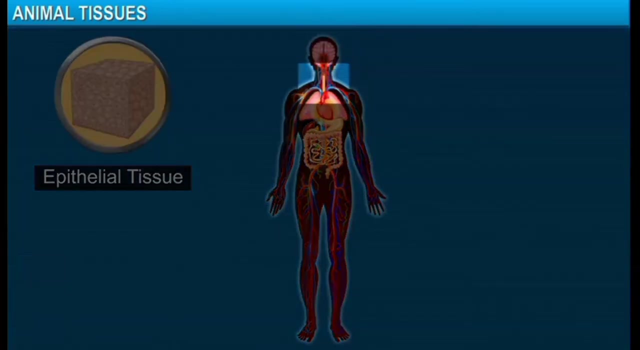 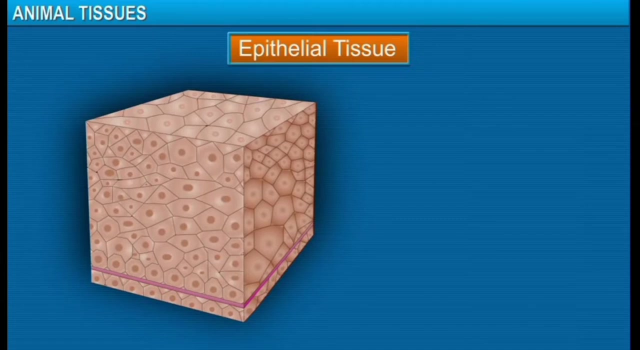 muscular tissue and nervous tissue. Let's look at each tissue in detail. Here is the epithelial tissue. These tissues form a protective layer for organs. Epithelial tissues act as a barrier to keep the different body systems separate. The epithelial tissues consist of closely packed cells without intercellular spaces. 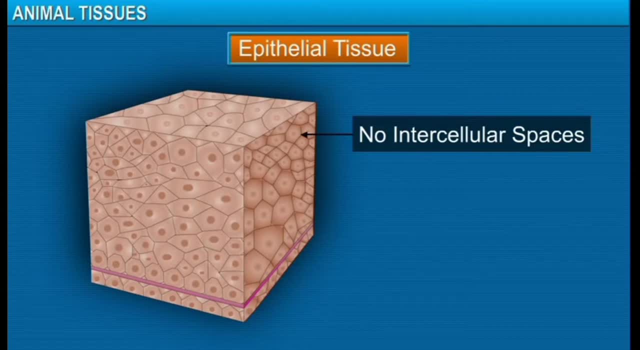 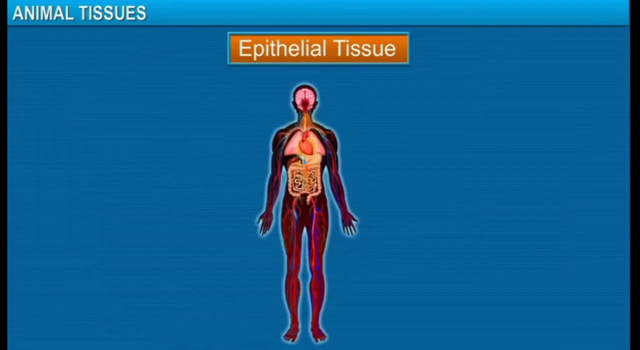 These tissues are separated from the underlying tissue. The tissue is divided into two sections. The Montargh tissues are different from the underlying tissue. The epithelial tissues are separated from the underlying tissue by an extracellular fibrous basement membrane. Epithelial tissues are of different types depending on their shape and function. 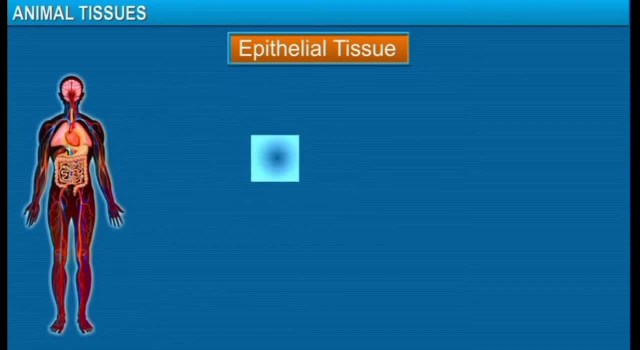 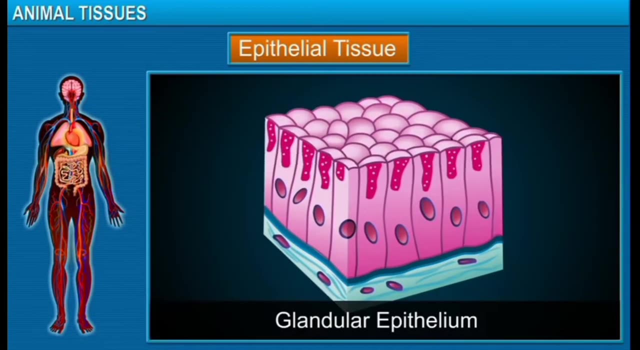 The different types of epithelial tissues are squamous epithelium, columnar epithelium, glandular epithelium, ciliated epithelium and closely linked epithelial tissues. To get more information, visit our website at wwwfemagov. You may also be interested in learning more about epithelial tissues. These tissues are made of different types of tissues. Parts of the epithelium are called epithelium, glandular epithelium, ciliated epithelium, calumnar, epithelium and polyp. 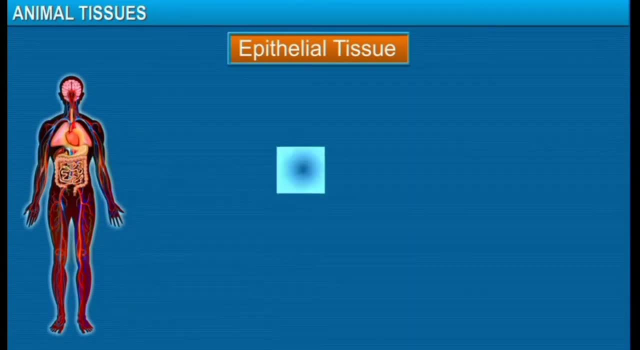 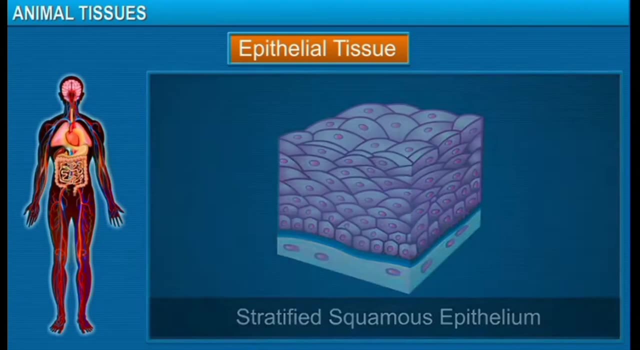 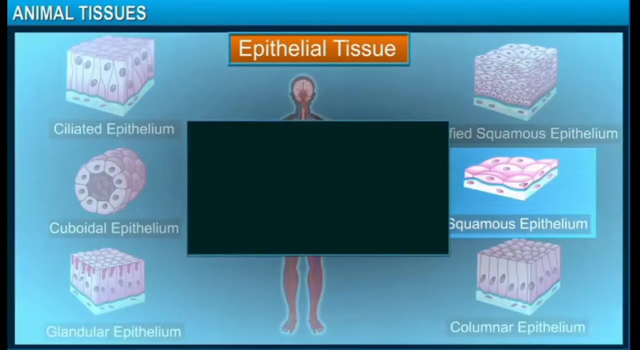 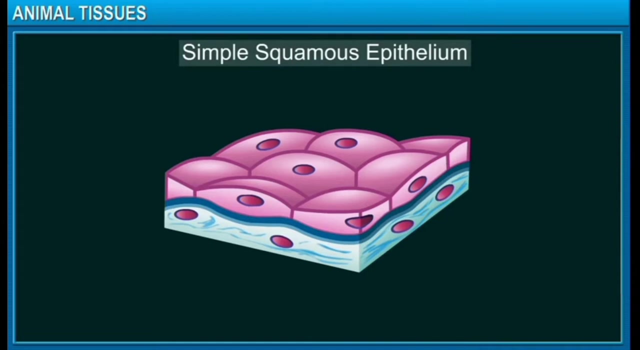 Celiated epithelium, cuboidal epithelium and stratified squamous epithelium. Let's first look at the squamous epithelium. The simple squamous epithelium has flat and thin cells. These cells group together and do not have intercellular spaces. 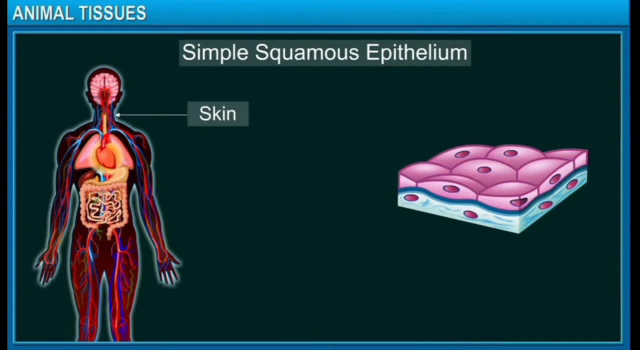 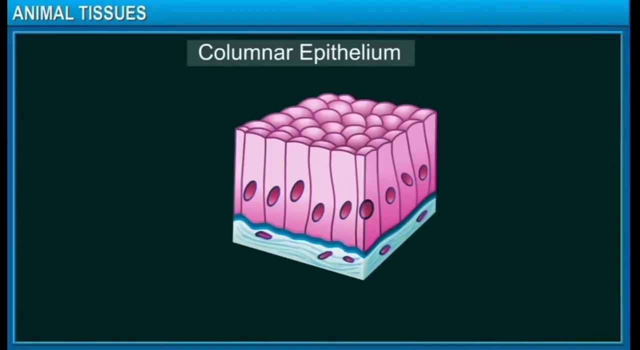 They are found in the outer layer of the skin lining the cavities of ducts, blood vessels, lung alveoli and the chambers of the heart, and provide mechanical support. These pillar-like cells are called columnar epithelium.